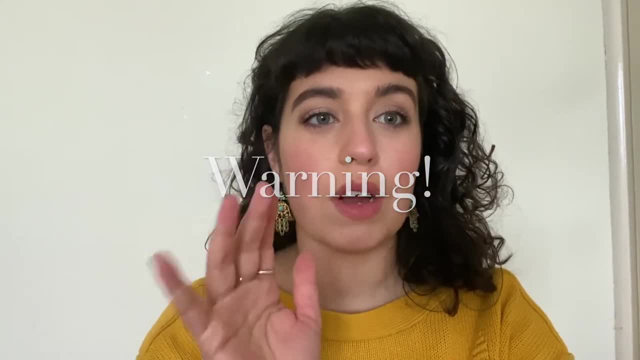 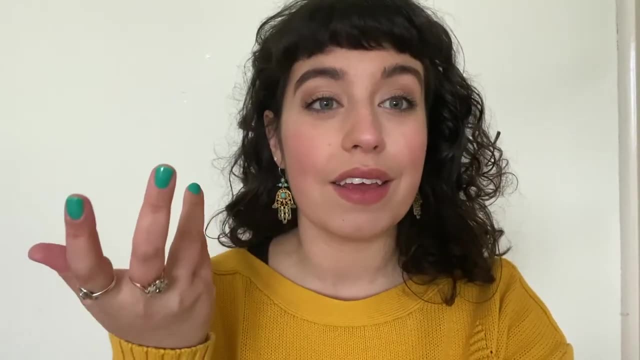 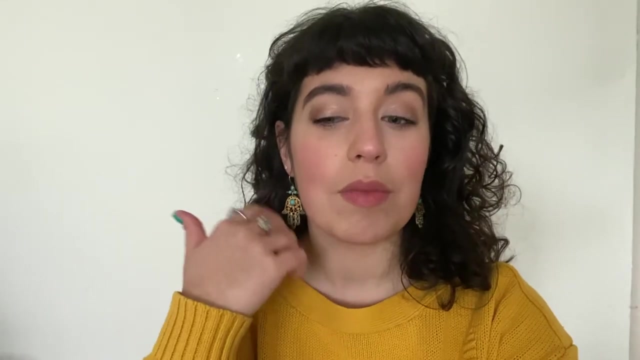 Just a really quick word of warning before you start this video. You need to make sure you have an adult supervising you when you're using the. you'll be using the stove on an oven which is hot, so you need to be really careful and have someone watching you all times and at the end you need to. 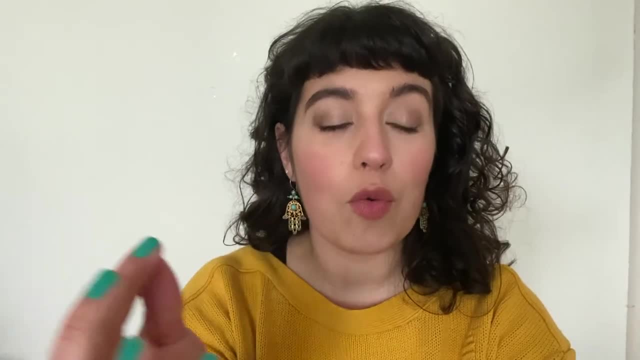 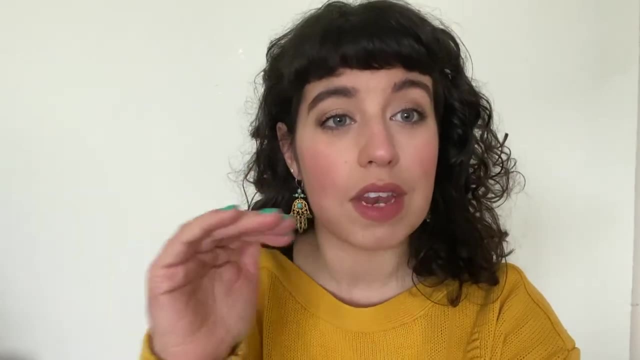 ask an adult to take the tin foil off of the saucepan because it'll be really hot. You have to make sure the saucepan is cooled down because the steam from underneath the tin foil lid that you're going to create will be really, really hot, and I don't want any of you. 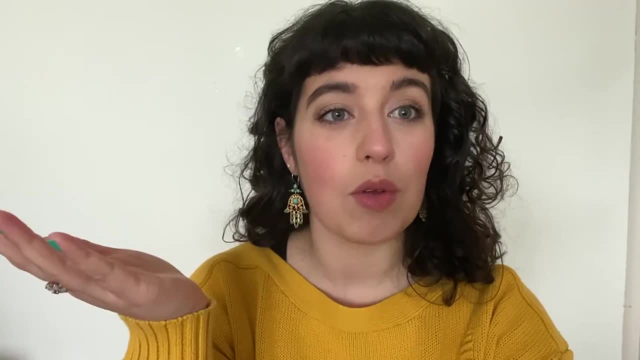 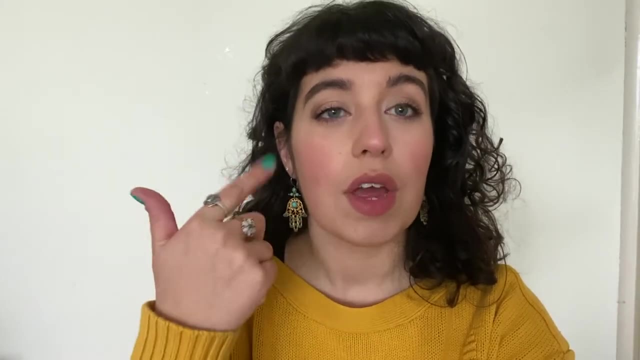 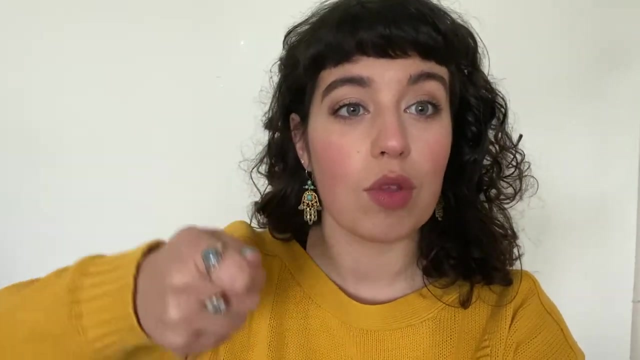 burning yourselves. Anyway, that's just a quick word of warning. so an adult supervising making sure that you're careful with the stove and that you're really careful at the end that you don't lift off, you don't get tempted to rip off that tin foil straight away. You wait for it to cool down. 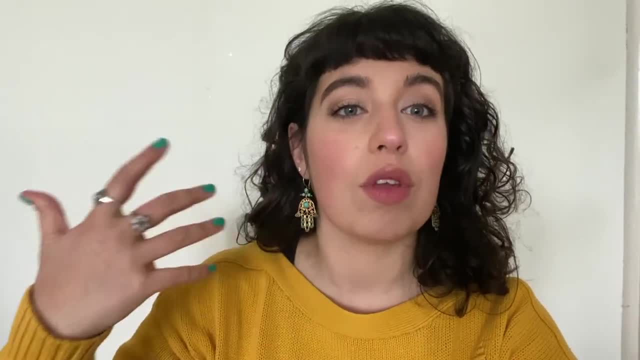 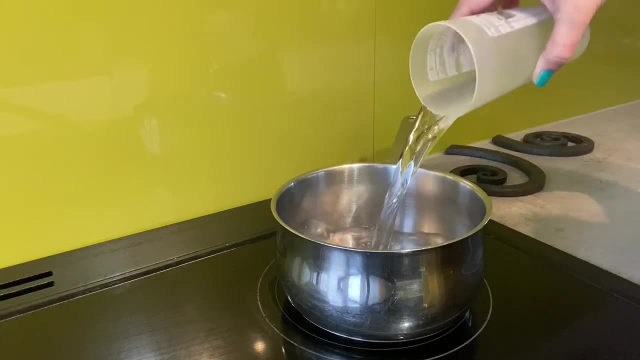 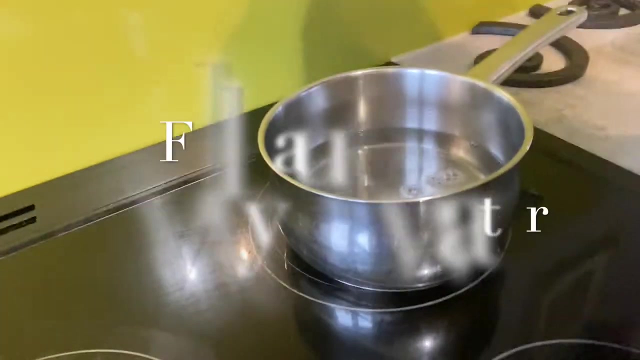 you wait for that water to cool, That saucepan to cool, and then you can take off the lid. That's it. Have fun with this experiment. Right, hello, Year 5 welcome. So we are imagining the stove, is the earth creating heat and you're. 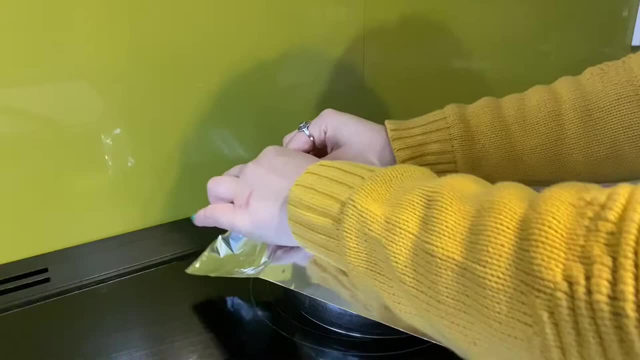 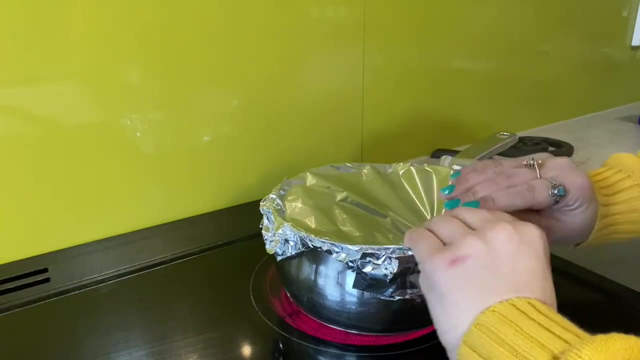 going to want to put it on a medium heat- imagining the earth is a medium heat- and cover it just halfway. Then I grabbed some foil and I placed it on top, curling it over the edges, making sure that the heat is going to be on the top. So I'm going to put it on the top and then I'm going to. 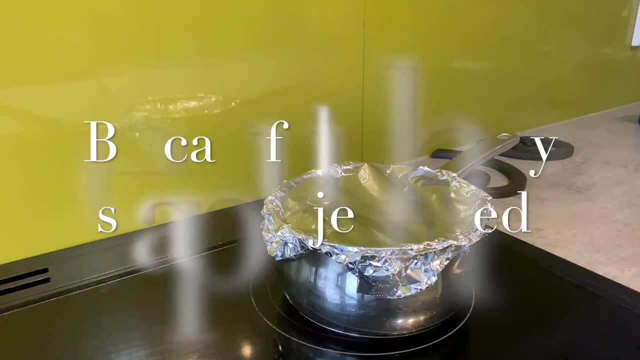 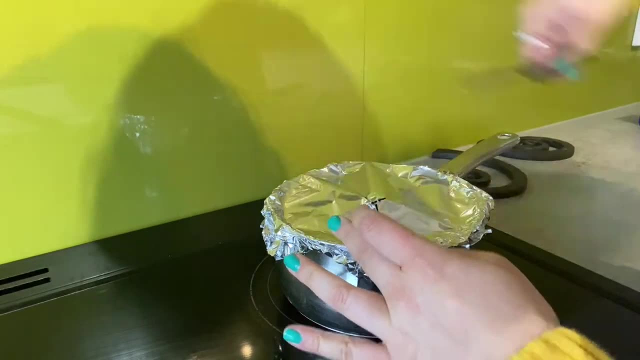 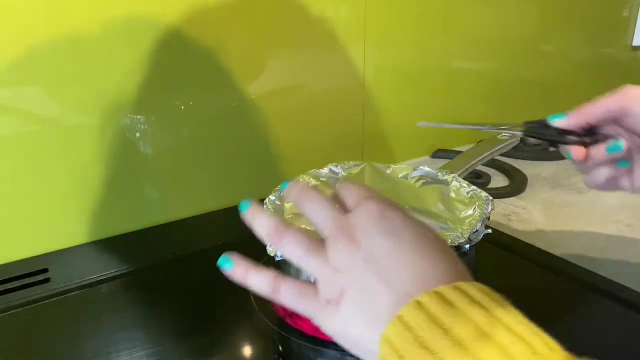 put it on the bottom of the stove. I'm going to put it on the bottom of the stove so it didn't catch, and then I just use my scissors to create an insertion at the top. Okay, so you're imagining that the foil is the earth's surface and that tiny hole is where all of the pressure from the heat. 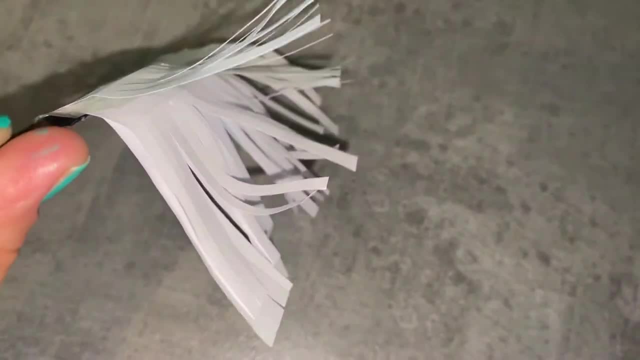 is trying to escape from. I then wanted to create a paper fan. Basically, I know you guys won't have pins on your paper, but you can use a paper fan to create a paper fan. So I'm going to put it on the top and then I pressed on it so it would slide out of the frame. I'm going to use a bit more pressure. 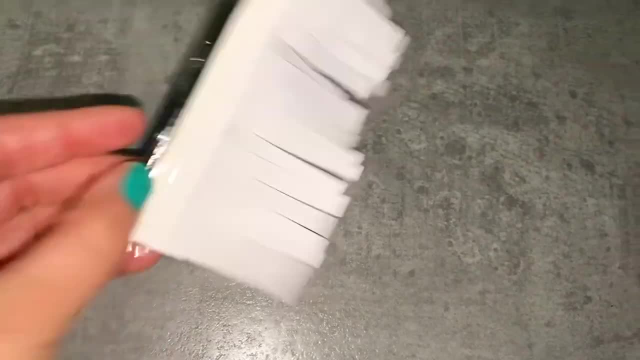 and then I'm going to take a bit of tin foil to create a windmill. Now I'm going to tell you a bit more about the windmill. It's a little more powerful than the windmill. It's a little more powerful and it's pretty convenient to use, but I am not going to use it very much. You could take.